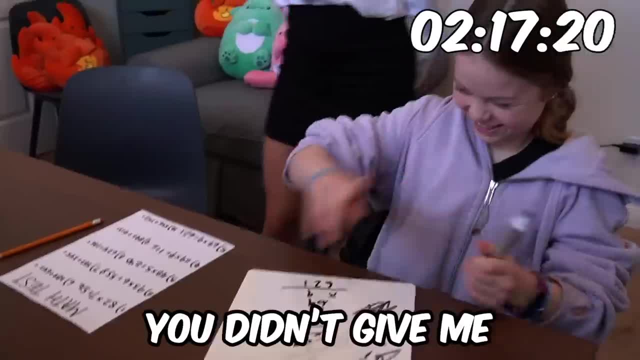 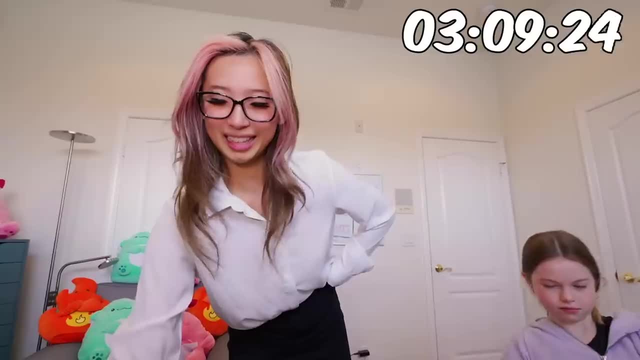 a lot to learn. Michelle, give me an eraser. One hour is gonna be hard. I'm only in seventh grade. How am I supposed to know these off the top of my head? And time Three minutes and ten seconds. So this one's wrong. Oh no, This one is close. What? 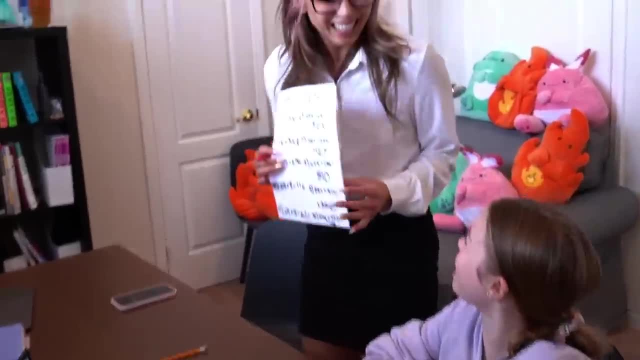 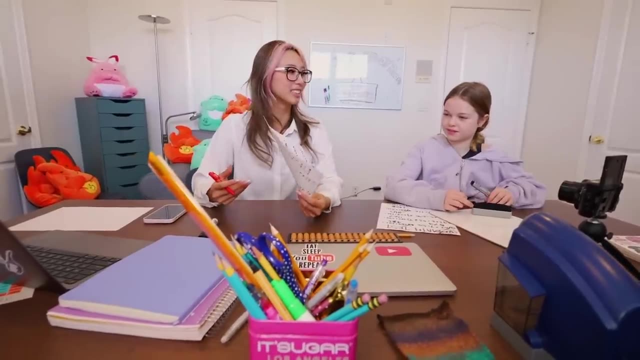 That's not bad. That's so bad. It's like the worst grade I've ever gotten. It's a 70 percent, But you did it in three minutes and ten seconds. Oh, We can do better. Let me show you how fast. 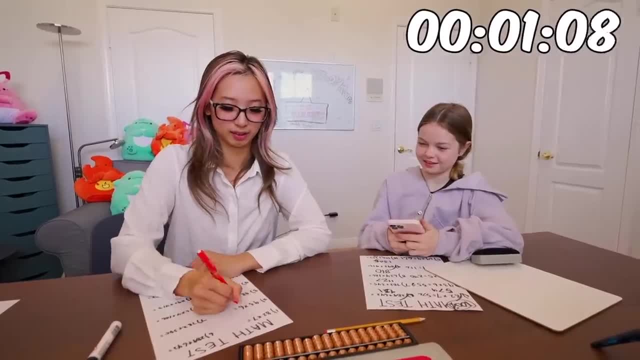 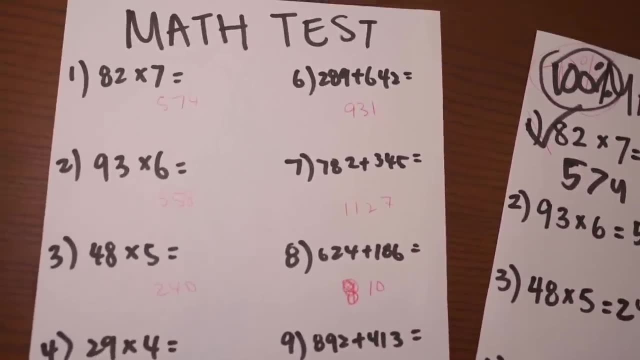 you can do this once you learn my secret. What, Wait, how I'm done. 20 seconds, I mean she did okay. 70 percent is still passing, but I think we can speed up the time a little bit. 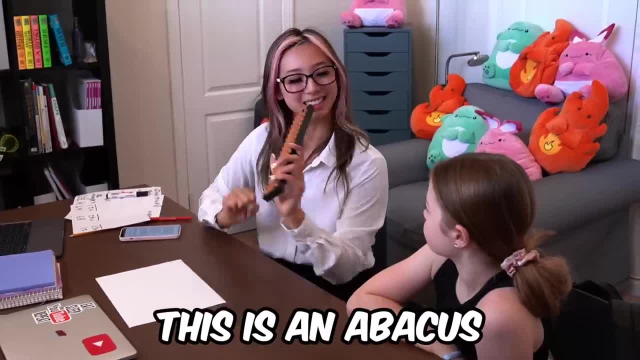 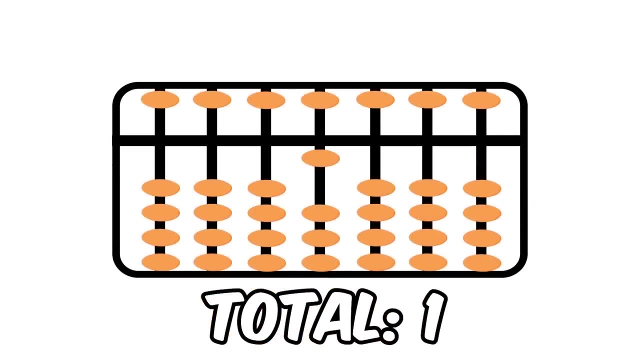 So, first period, we are going to learn speed. This is an abacus. This is how I learned to do math. Yeah, you can play with it. These speeds go from one all the way to nine. There's five, Yes. 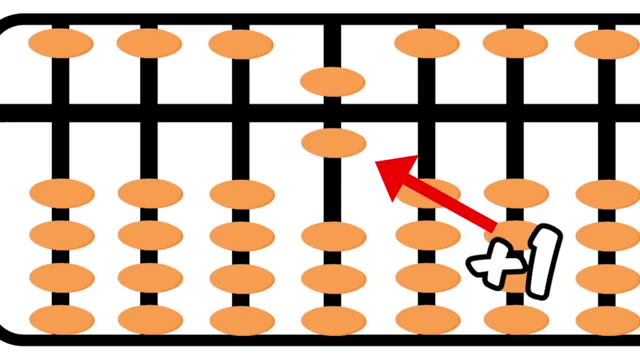 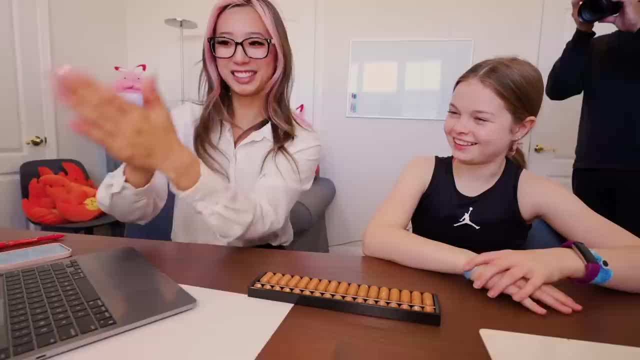 So the top is five, This is six, This is seven, This is eight, This is nine. This is the rules of the abacus. These are the small friend formulas. So for number one, the small friend is four. For two it's three, For three it's two And for four it's one. What It's four? It's one. 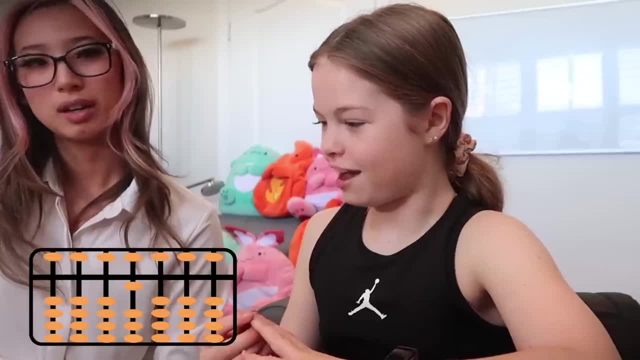 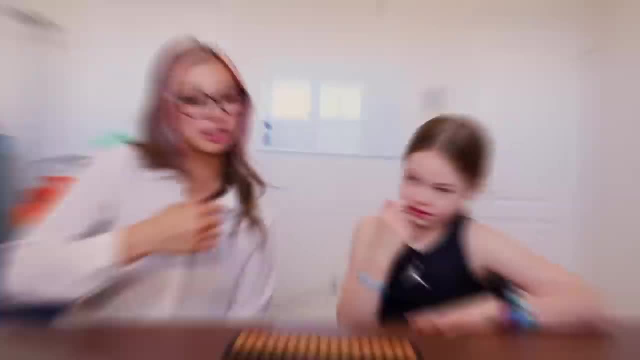 If you want to do one plus four, one. No, that's five Five, five minus one. Oh yeah, that makes a lot of sense. I'm so confused I don't think I'm a very good teacher. So this is the ones digit, right? 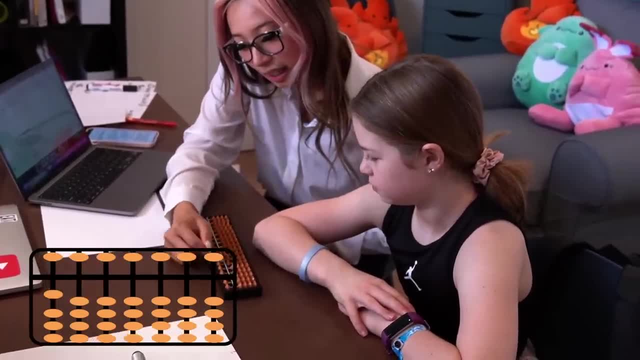 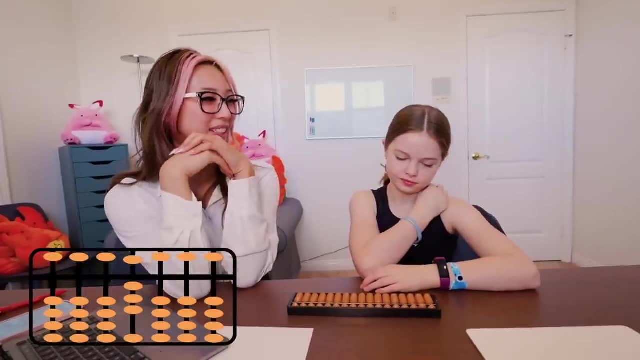 here, the stars. This is one, This is ten, a hundred, a thousand, What? And this is like a million. Yeah, this is a million. Okay, I got it. Okay, it's clicking Three plus three on the abacus. 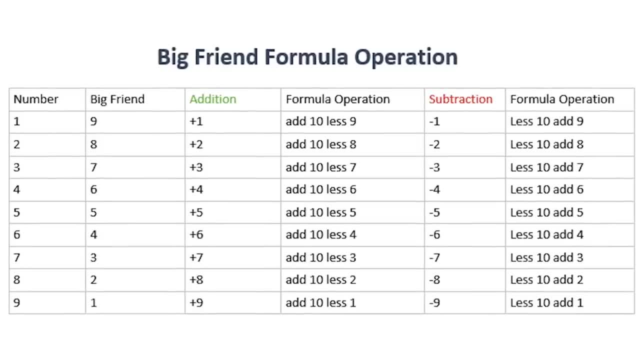 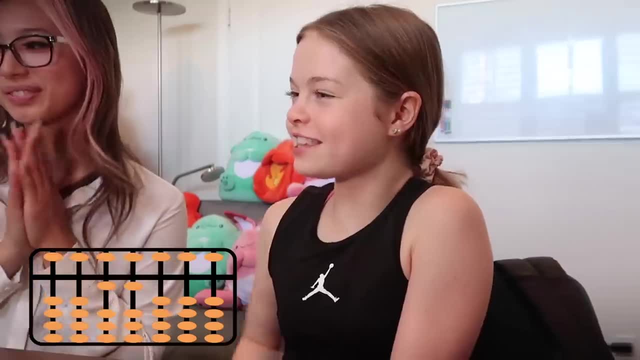 Right, but how would you show your work? You have to show it, Big friend. formula is also very easy: Four plus seven Eleven. Add ten minus three. Four plus seven is eleven, Yeah. So then why am I adding subtraction? That's just the rules of the abacus. I think you got the hang of it. 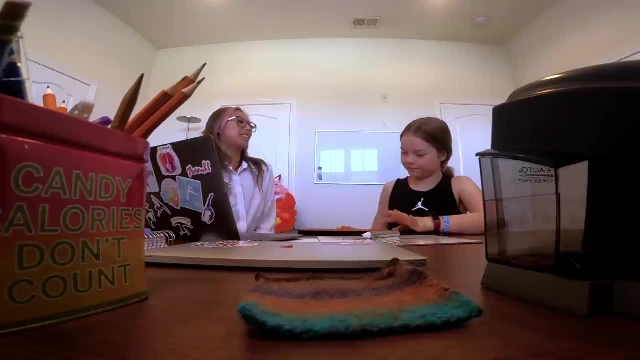 Yeah, you got it. Yeah, I think she's got the hang of it. We can take the first test for period one. Wait, there's a test. You're gonna answer these flashcards in 60 seconds as fast as you can. Three: 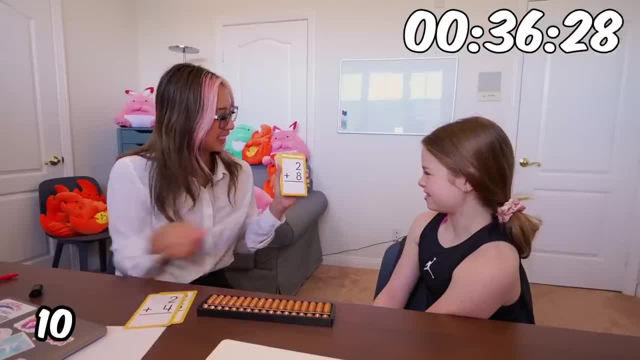 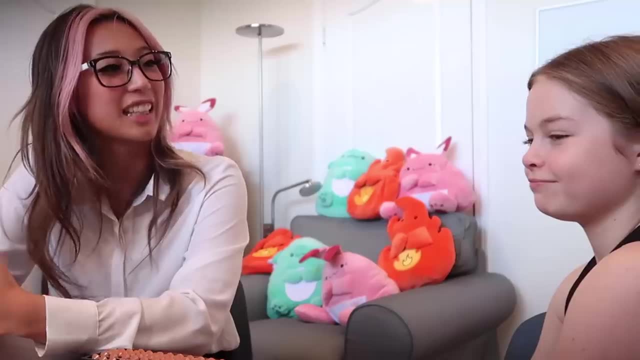 two, one go, Five, six Nice, Seven Nice, Ten Nice, Thirteen, Fourteen, Sixteen, One more, Four Nice. That looks pretty fast. I think you're ready for period two. Okay, Michelle, I don't know how you're doing, I mean, 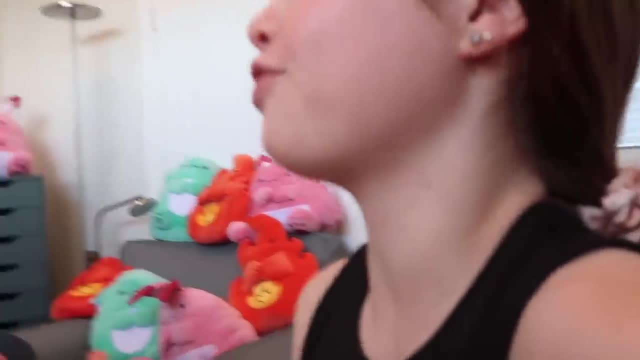 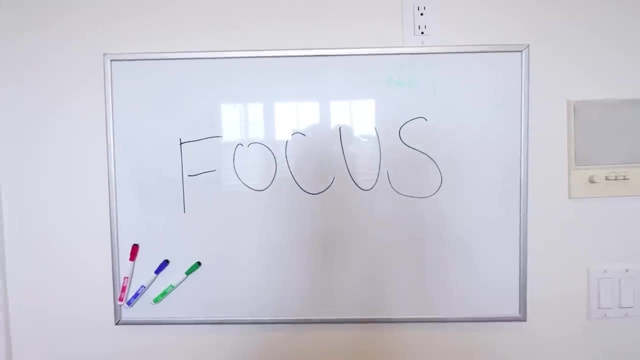 I think you're doing pretty well, but like I don't know if it's me or if you're just a not great teacher. Oh well, we have 45 more minutes to keep going For round two. you're gonna learn how to focus. I know how to focus As a human calculator. people are gonna. 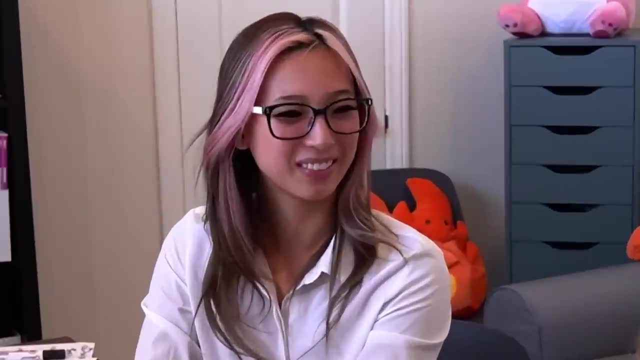 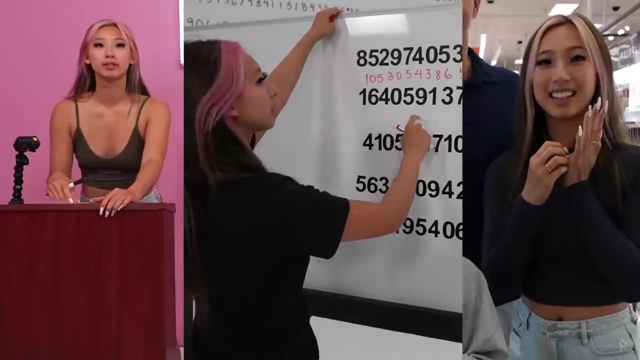 distract you. You are going to do jumping jacks while doing that. What? As a human calculator, you're gonna be distracted. and for me- you can see me doing this in other videos, where I look at my hand and imagine an abacus on my hand, and that's what helps me concentrate. so that's why I'm gonna 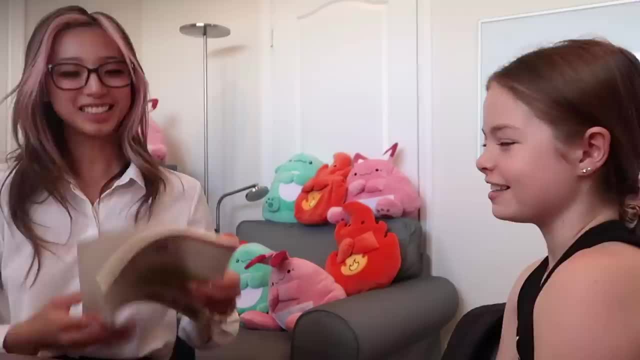 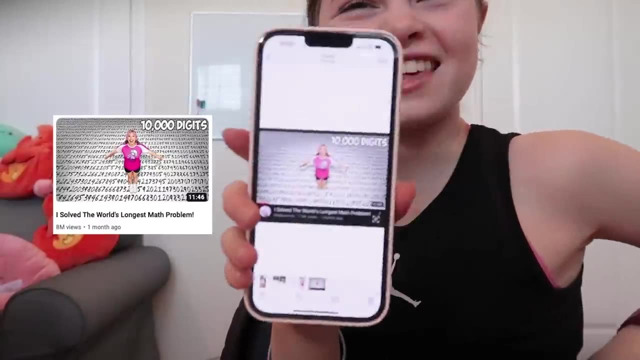 teach Salish today. Did you do your homework yet? What homework, This homework? It's our first day. Okay, this is what I learned in class, This is what I have for homework and this is the test. You're gonna do flashcards while doing jumping jacks. Let's get it started Now. 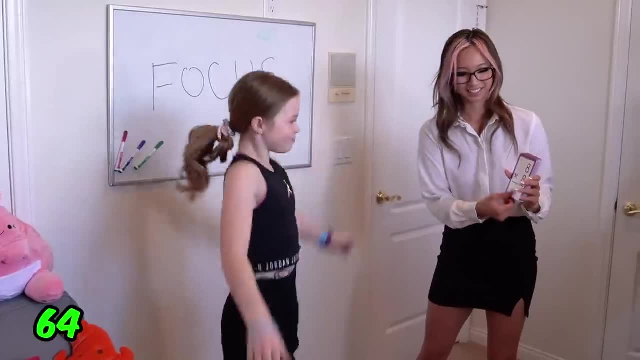 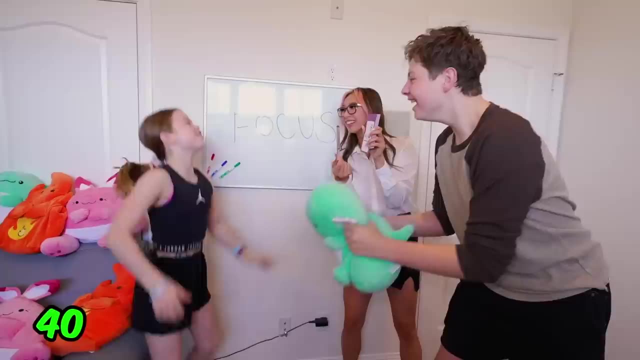 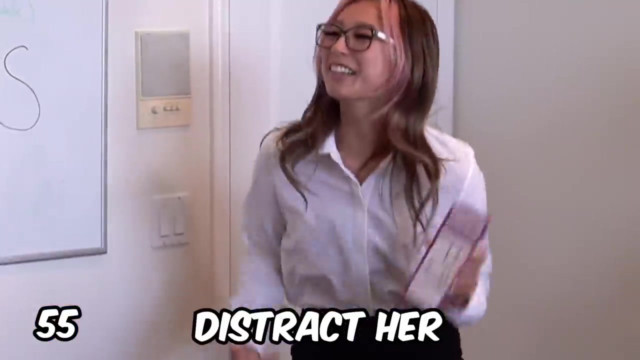 try and answer these math questions: 22,, 80,, 72,, 64.. Now we're gonna add on some real distraction. Hudson, All right, say: go Go. Oh, you suck, Answer the question. You suck 40.. You suck 8 times 2.. 8 times 3.. 21.. 8 times 0.. 0.. 88.. Distract her more, Hudson. 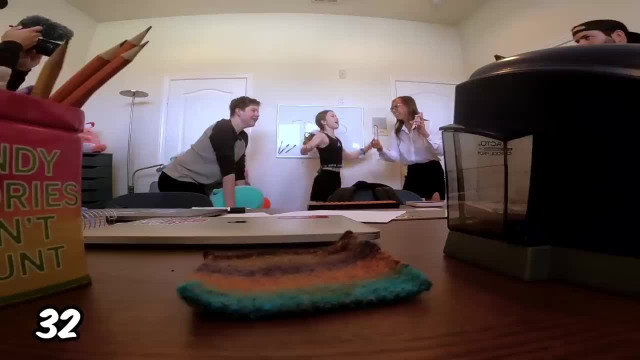 Salish? you suck. How's this? How's this? 76.. Come on, How are you Salish? you can't do it. You can't do it, You can't do it. 32., 32., 36., I don't know. 12 times 12.. Oh my goodness, I'm under. 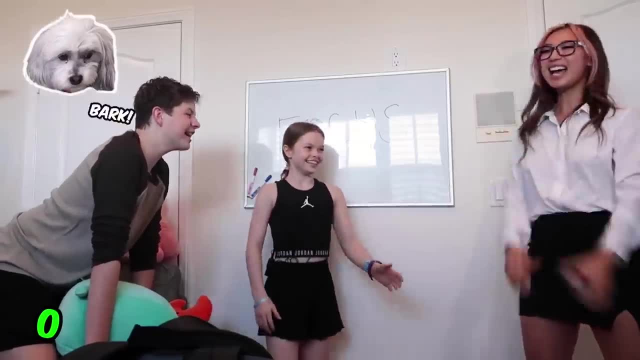 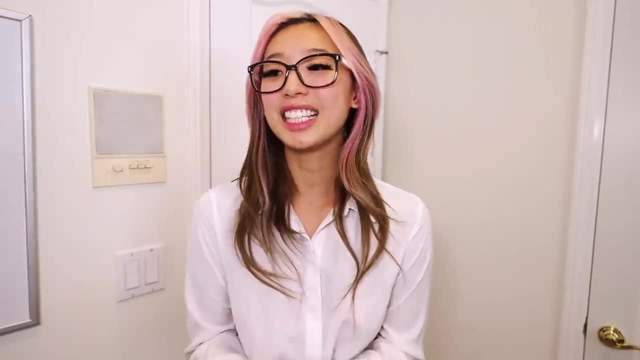 44.. 1. 21.. Last one: 0.. You suck, You suck. Oh sorry, Now I feel like you can do literally anything. Yeah, but those were easier than the test problem. Seems like Salish is a really really good student. 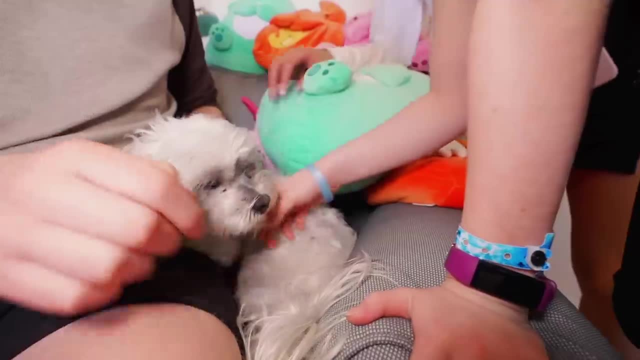 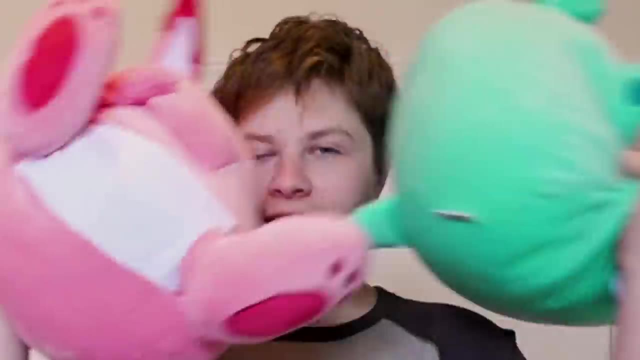 Action, however, did get to her a little bit. It looked like she was struggling, but eventually she pulled through. She probably looked faster than I would have done it. I'm very proud of the teacher. These are insanely fluffy. I mean like, make sure you guys go get these right now, Yeah. 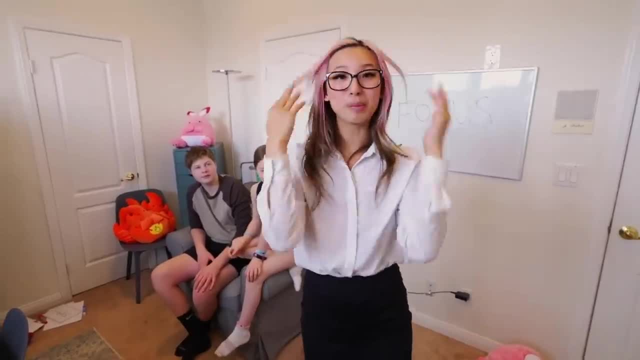 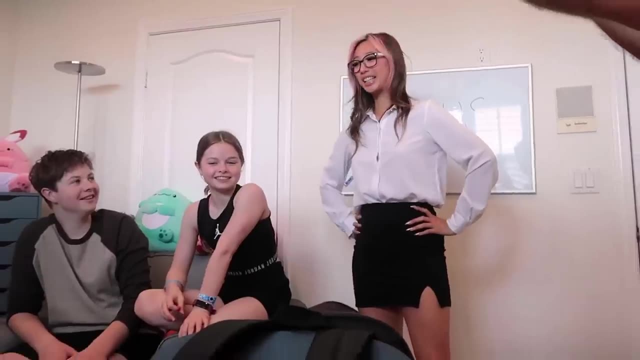 get these at zcstorecom. We have 30 more minutes. I have one more lesson left and I still have to give her a final test. What's the next lesson? Accuracy. What Accuracy, Being a human calculator? if you don't get these questions right, people will blame you in the comments. But before we do this, 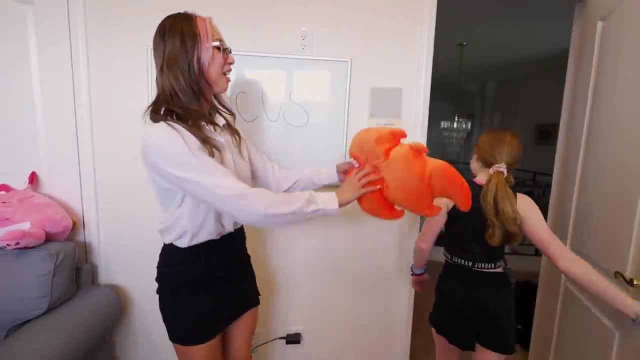 I'm going to teach you how to do multiplication on the abacus. Oh, do you want to do that? Sure, Recess, I'll see you in like never, Wait, wait, Take a hall pass with you. Oh, perfect, Thanks. 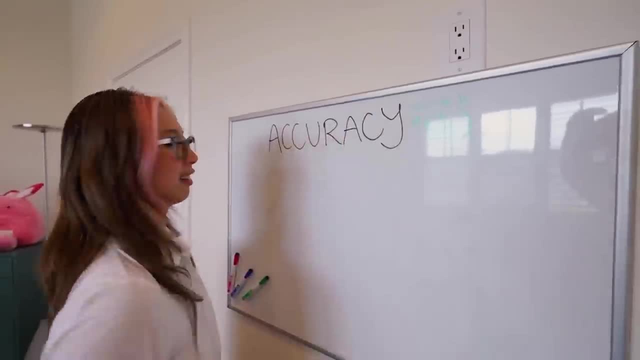 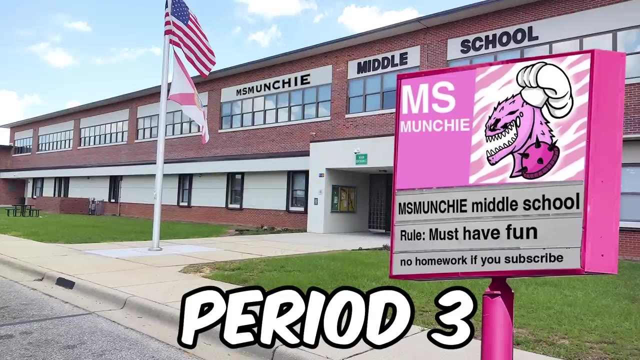 Wait, never. Teaching a kid to become a human calculator is way harder than I thought. I think she's doing great, though I really think I just need to build up her confidence and get her really comfortable with using the abacus. Every single problem you get right, I'll give you $20.. And if 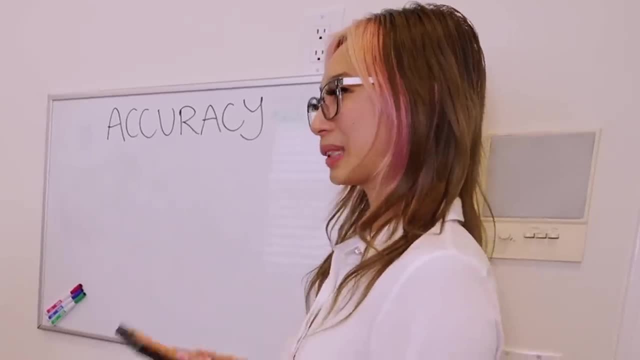 you get it wrong, you lose $100.. Before I give you the test, I'm going to teach you how to do the abacus. Oh no, So for the abacus, instead of going from right to left, you're going to go. 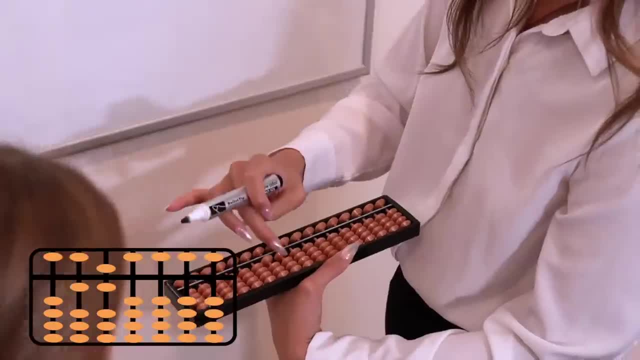 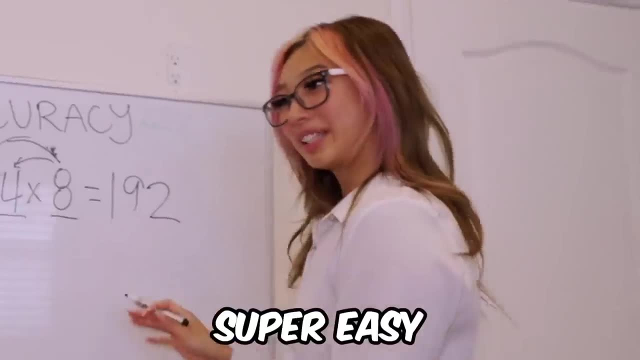 from left to right, What is eight times two, Sixteen, Sixteen, And then what's eight times four, Thirty-two, Can you add in thirty Two Hundred nine, two. Yeah, Super easy, Super easy. One, eight, nine, Yeah, I think she gets the hang of it and I'm actually very, very happy Time. 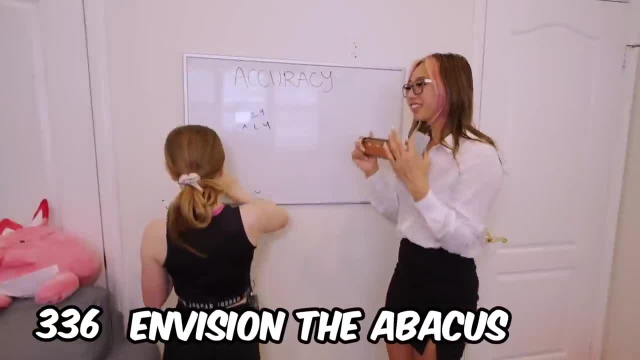 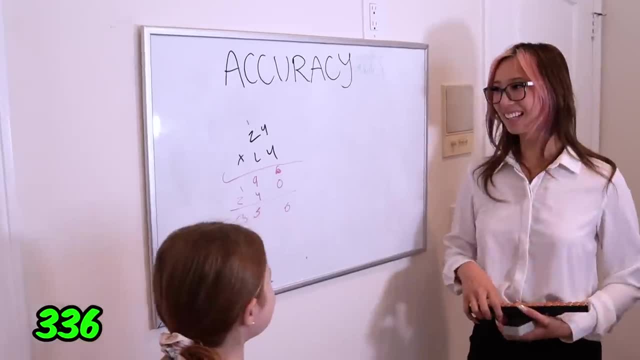 for the test. What's 24 times 14?? And remember, envision the abacus in your head: Four, eight, 12, three, one, three, Yes, Twenty dollars, Okay, Times eighteen. And then, if you do it on the abacus, 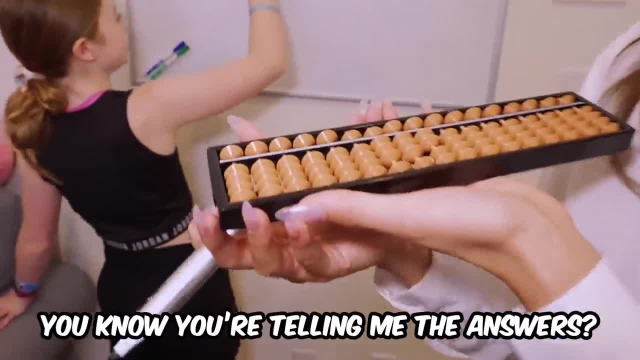 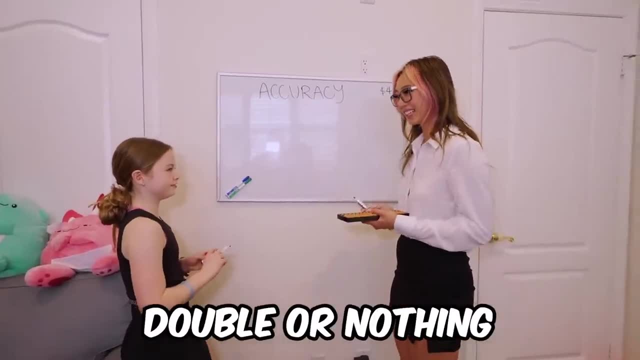 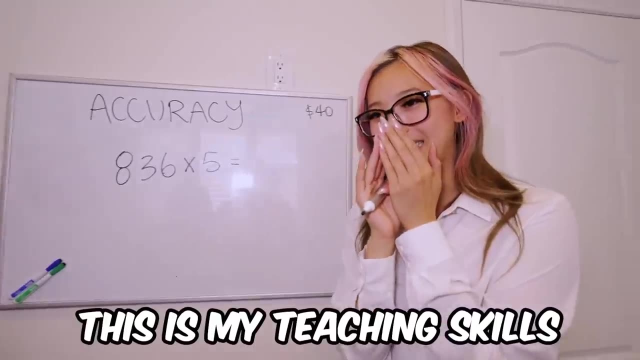 eight times four is thirty-two. So this is the answer. You know you're telling me the answers. Nice, Forty dollars. For the next question, I'm going to give you double or nothing, if you choose to use the abacus. Okay, How many is it? Eight hundred thirty-six times five. This is my. 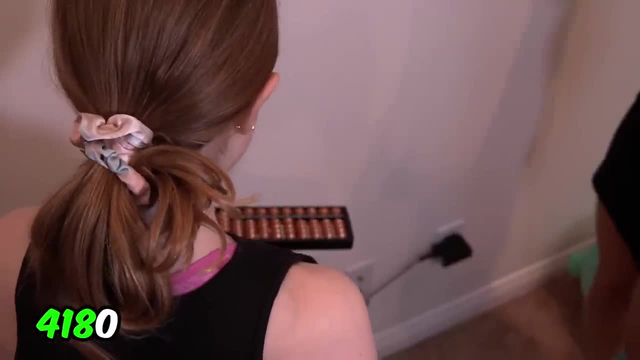 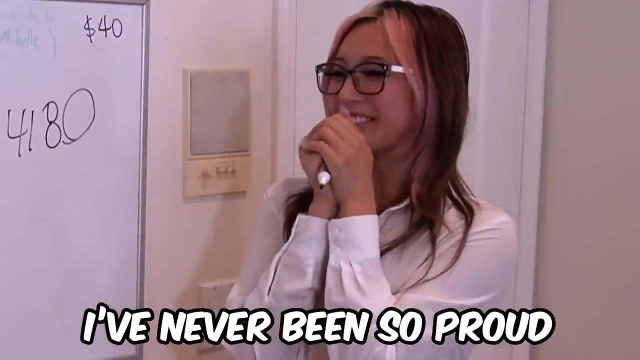 teaching skills put to the test. Four, one, eight, Yes, Zero. Did I get it? Yes, I got it. Oh my gosh, you learned how to use an abacus. I've never been so fast. Eighty dollars, Here I come. I can't believe. Salish learned how to use an abacus in less than. 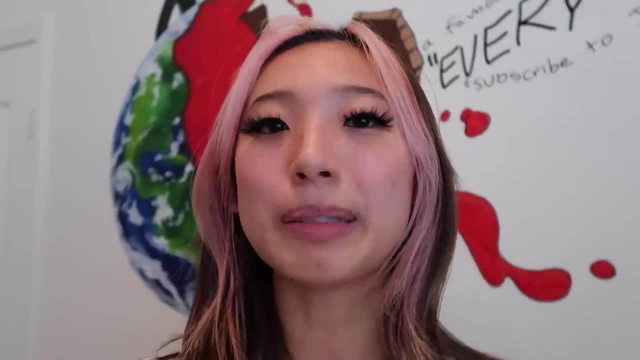 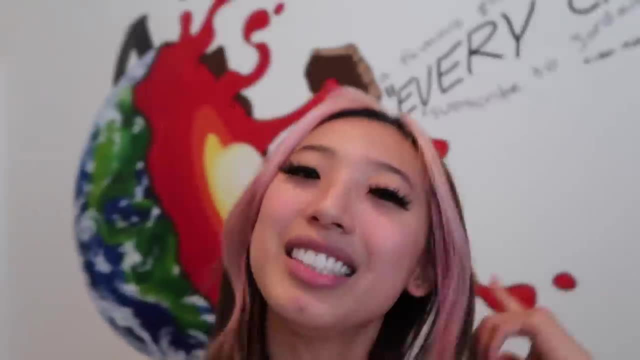 an hour. She completed the math problem and she got it right, And I hope this inspires you guys to keep practicing and keep working hard. Even if you fail the first few times, eventually you're going to get it right. Also, isn't this super, super cute? Zach and I customized this room for 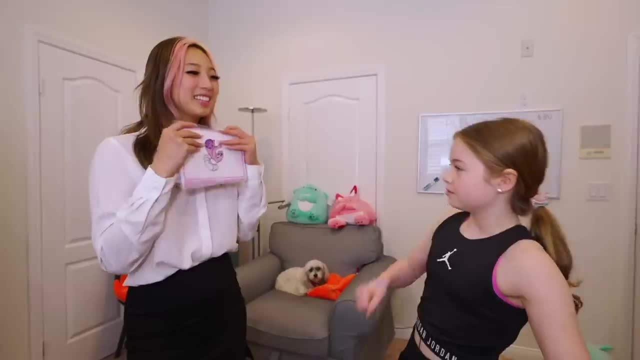 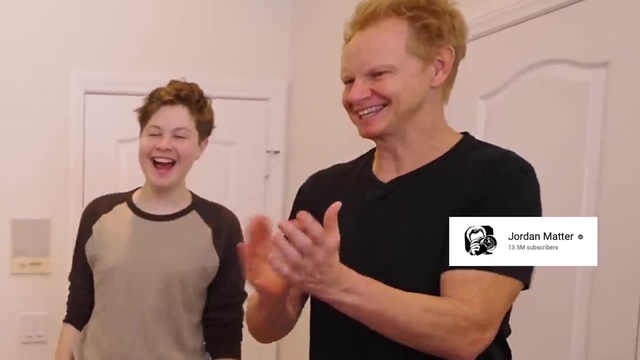 Salish and you can see it in this video right here, And I'm going to show you how to do it Right here. Now it's time for your final math test. Okay, I brought your dad and your brother along And just to show you guys how far she's come. this is her original math test Seventy. 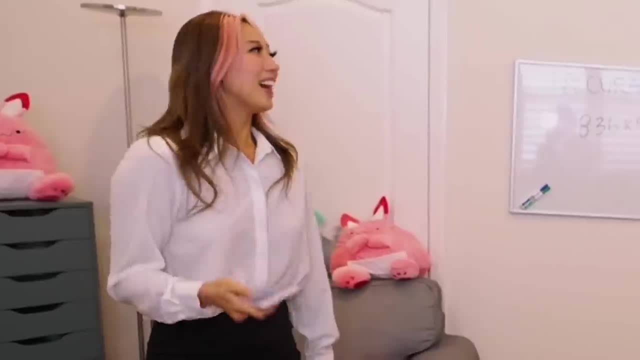 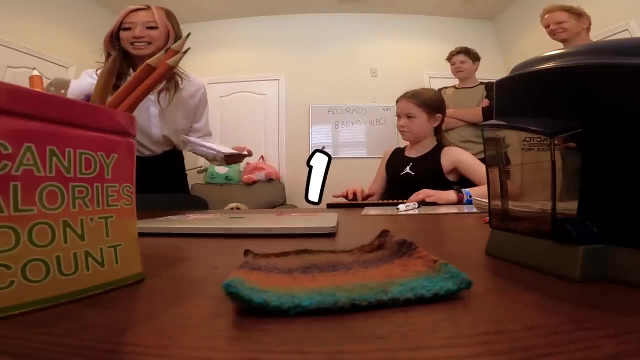 percent, three minutes, You got this. All you need is a seventy-one percent. Wow, why am I nervous? Please do well, This will prove that I am a good teacher. Three, two, one go. Twenty-four times eight. Two, twenty-eight, sixteen, Eight times four. thirty-two, Three. 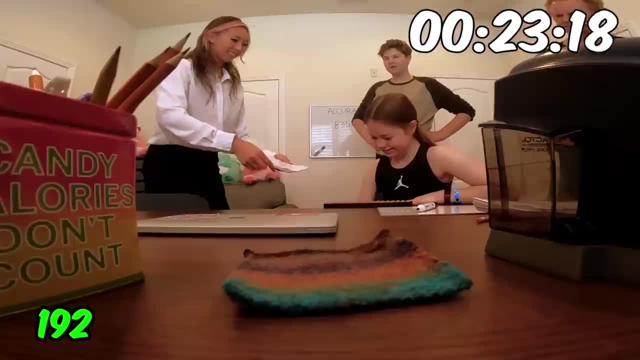 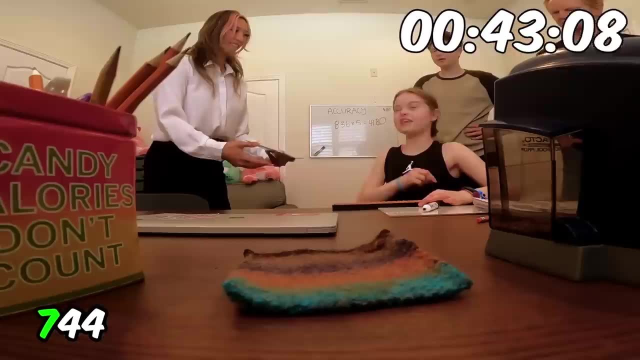 two, one, five, nine, two, Yes, Ninety-three times eight, Eighty times nine, seventy-two. I have absolutely no idea what she's doing right now. Two, four, Seven hundred and forty-four. Whoa, That was a lot faster than I thought. Yeah, Forty-three times three, Four, eight. 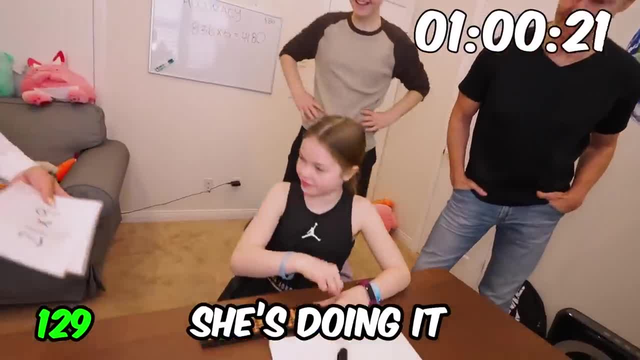 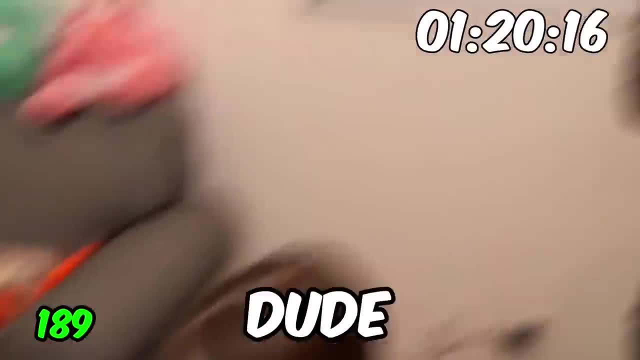 twelve, One, twenty-nine, Yes, Oh my gosh, you're doing it so fast. Twenty-one times, nine, Eighteen, Twenty-seven, No Hudson, no One. eighty-nine, Yes, Dude, wow, Seventy-two times. 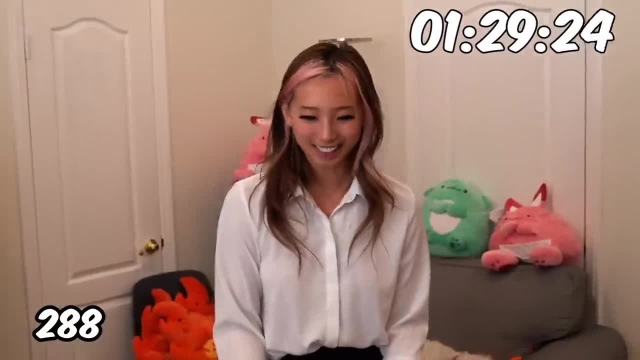 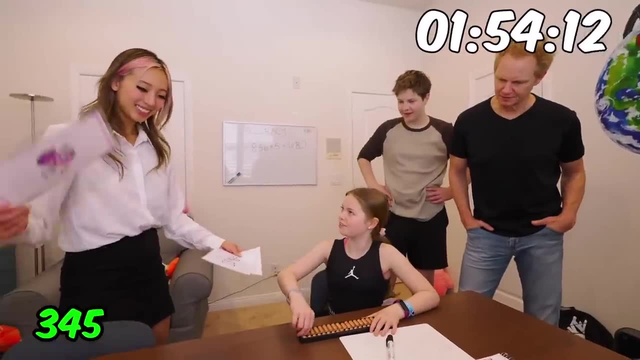 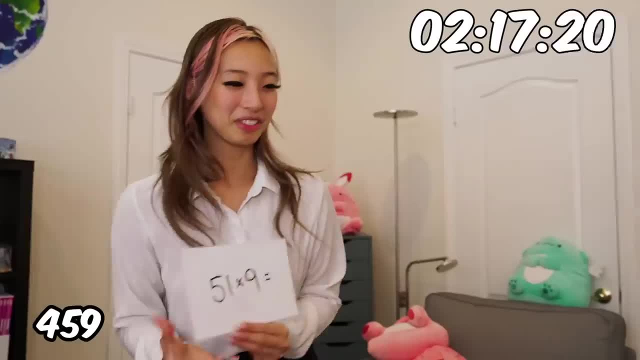 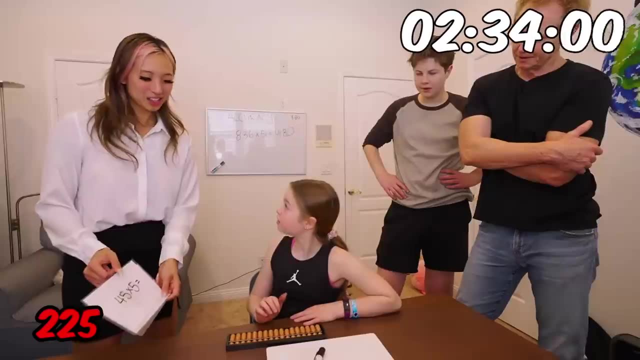 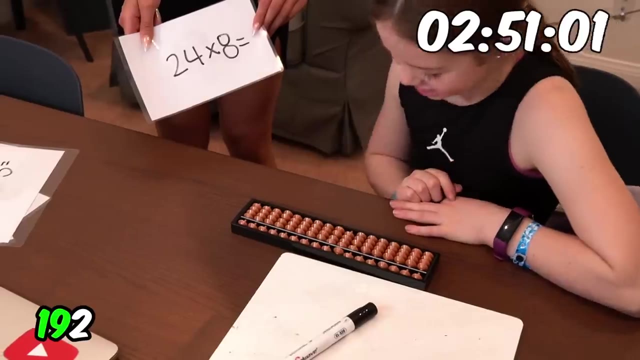 proud. I can't believe you understand this. One-ninety-eight, Yes, Fifty-one times nine. Four-fifty-nine, Yes, Forty-five times five. Five times five. Oh close, It's not four-fifty, Okay, whatever, I got to go. Twenty-four times eight. One, nine, two. 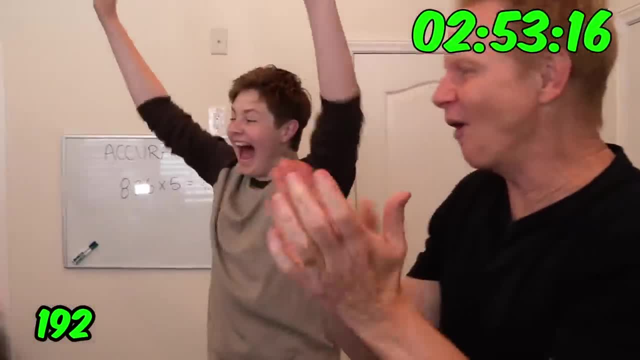 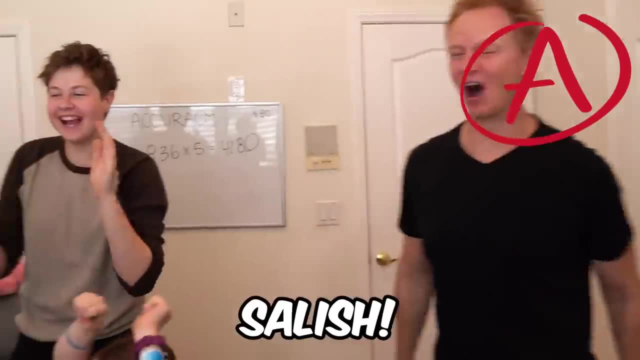 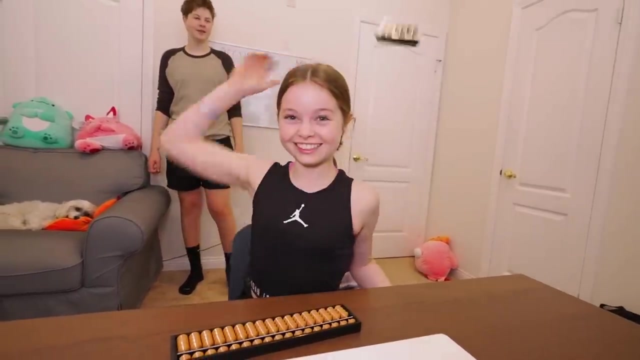 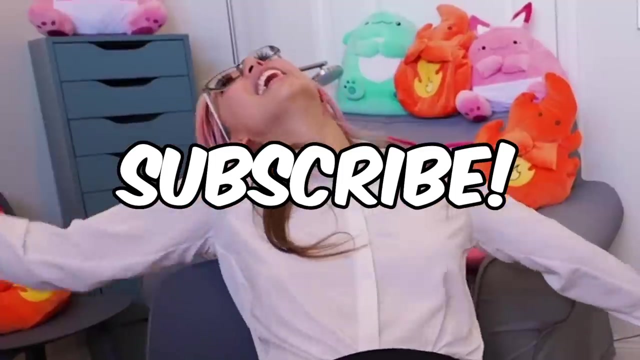 one-ninety-six. Go subscribe right now to Michelle. So she got ninety-percent, right Ninety-percent, And she beat her time. I guess I don't need this anymore. Ten plus two: Wait, that's a fifty. All of these are five. you said, Um, yes, Am I just a bad teacher?